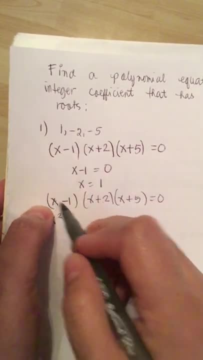 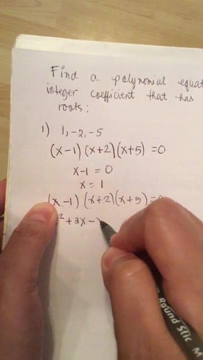 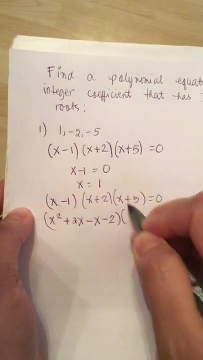 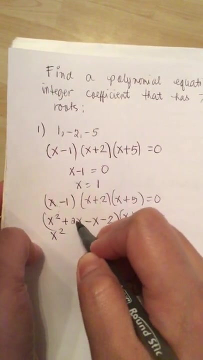 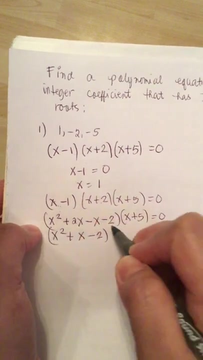 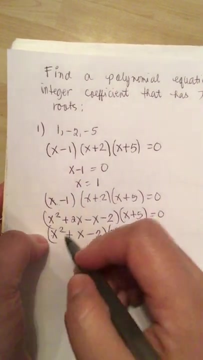 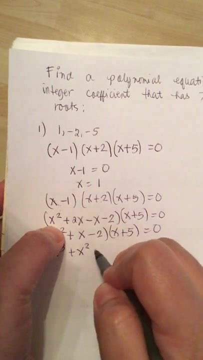 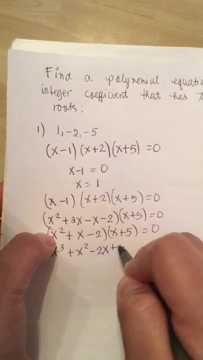 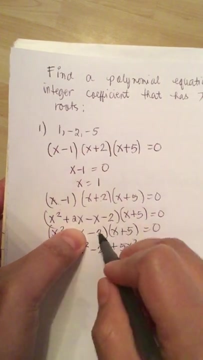 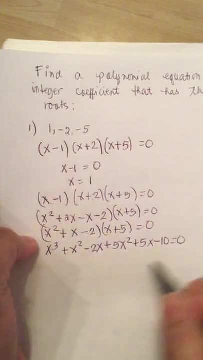 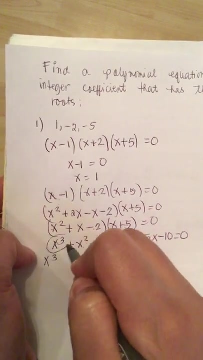 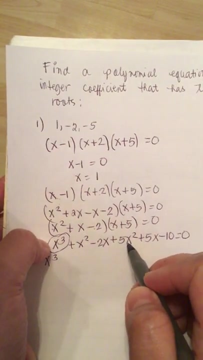 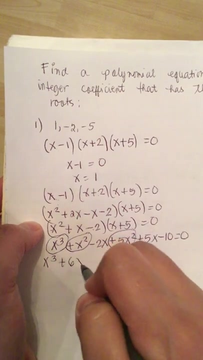 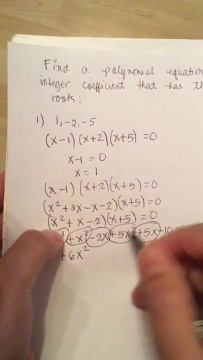 minus 2 is a minus 10 equals 0. so now we combine like terms. we have an x squared, so i circle that. so now we have an x squared plus 5x squared for a net of 6 squared. so now we have a minus 2x and a plus 5x for a net of plus 3x. now we have this minus 10. 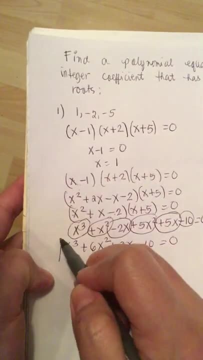 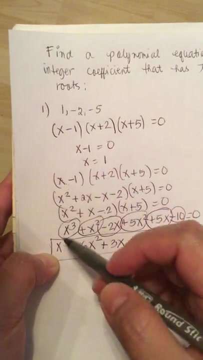 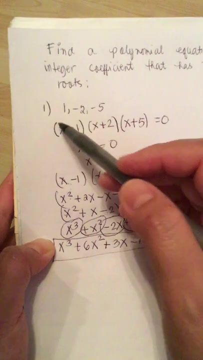 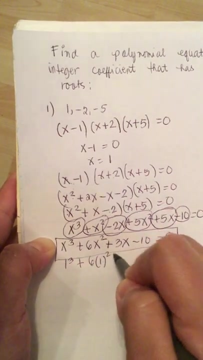 now equals 0. now, this is the polynomial that we're looking for. so now, if we substitute the numbers like the 1 minus 2 and minus 5, 1, We should get 0.. So let's try substituting 1.. So we have a 1 cubed plus 6 times 1 squared, plus 3 times 1 minus 10.. 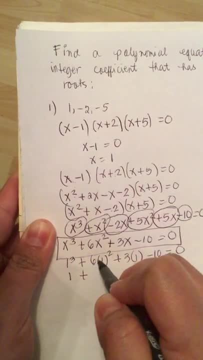 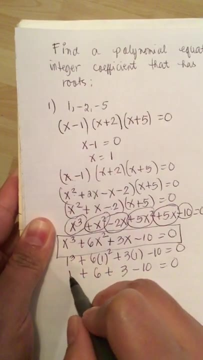 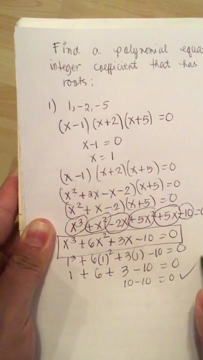 Does it equal to 0?? So this is 1 plus 6 plus 3 minus 10 equals 0.. So 1 plus 6 is 7 plus 3 is 10.. 10 minus 10 is indeed 0..